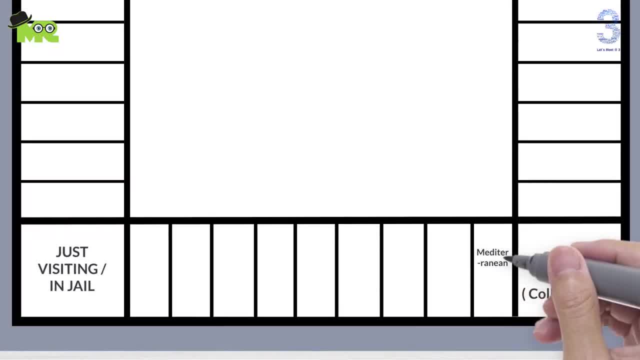 to the just visiting square. Write Mediterranean Avenue: $60,. here Community chest. here Baltimore Atlantic Avenue. here: $60.. Income tax pay: $200,. here Reading Railroad: $200,. here Oriental Avenue: $100,. here Write Chance and make a question mark. here Write Vermont Avenue. 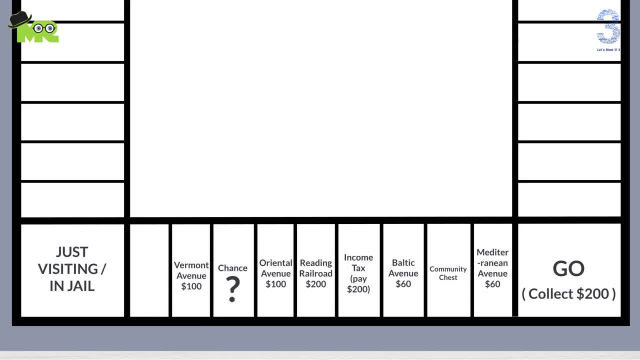 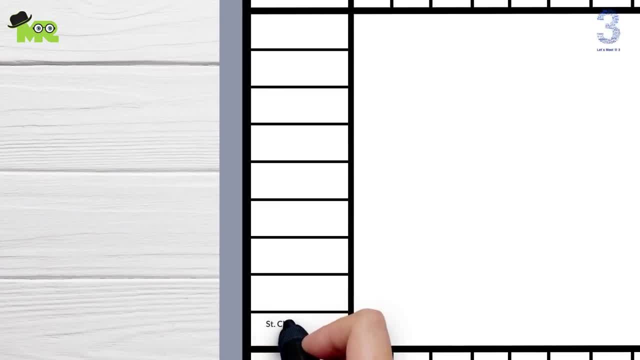 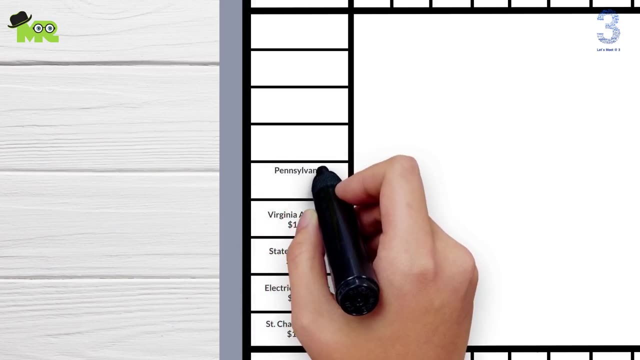 $100, here And Connecticut Avenue $120, here. Now let's label the side from just visiting to the free parking square. Write St Charles Place $140,. here Electric Company $150,. here, State's Avenue: $140,. here, Virginia Avenue: $160,. here, Pennsylvania Railroad $200,. 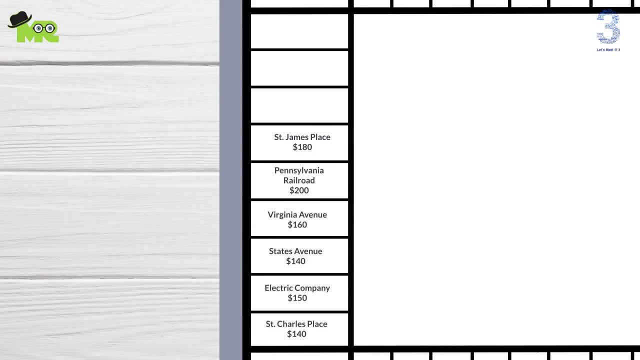 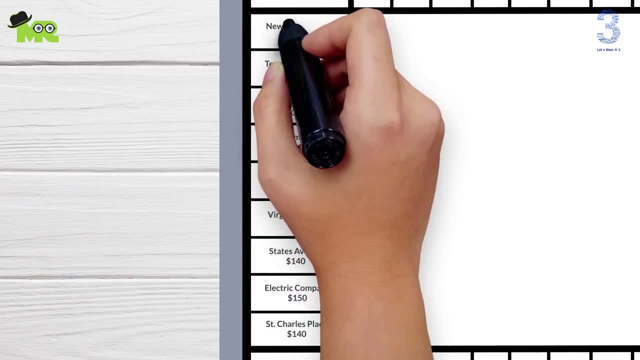 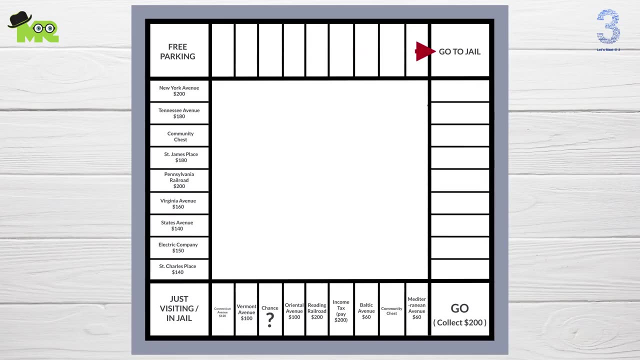 here St James Place: $180, here, Community chest. here Tennessee Avenue: $180, here. And New York Avenue: $200, here. Now let's label from the free parking square to the go to jail. 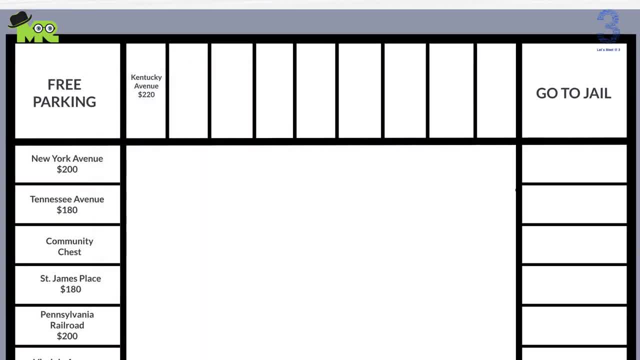 right: Kentucky Avenue: $220,. here Write Chance and make a question mark. here Write Indiana Avenue: $220, here Illinois Avenue: $240, here B&O Railroad: $200, here Atlantic. 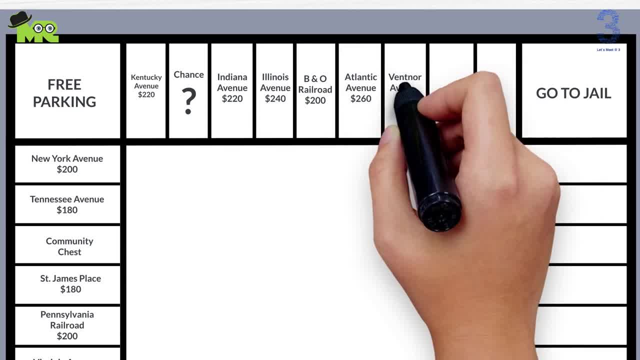 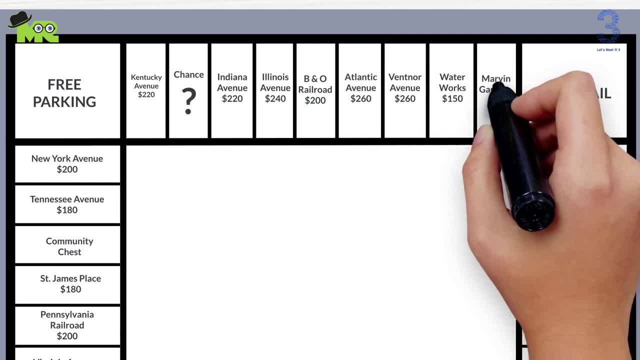 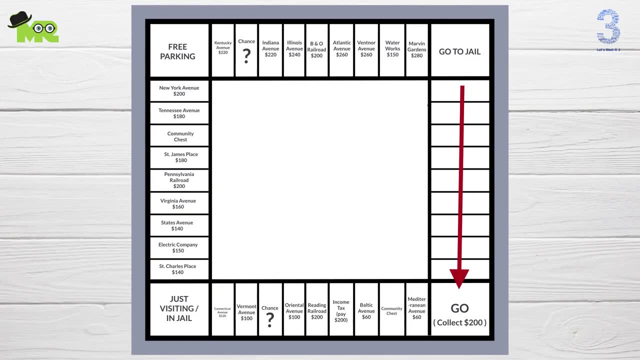 Avenue $260, here. Ventnor Avenue: $260, here. Waterworks: $150, here. And Marvin Gardens: $280, here. Now let's finish. the four side labels from go to jail to the go square Write. 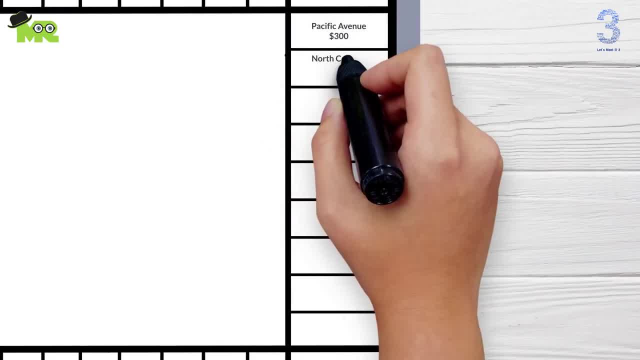 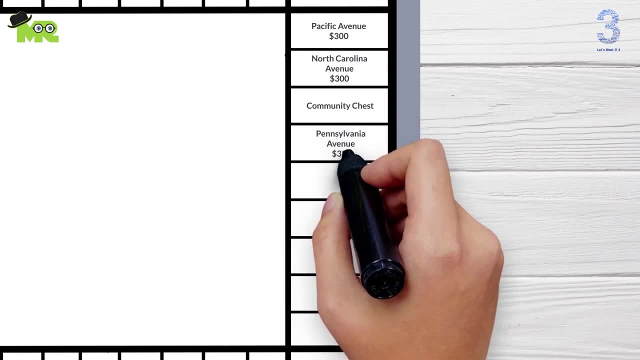 Pacific Avenue: $300, here North Carolina Avenue: $300, here Community chest. here Pennsylvania Avenue: $320, here Short line: $200,. here Write Chance and make a question mark here Write. 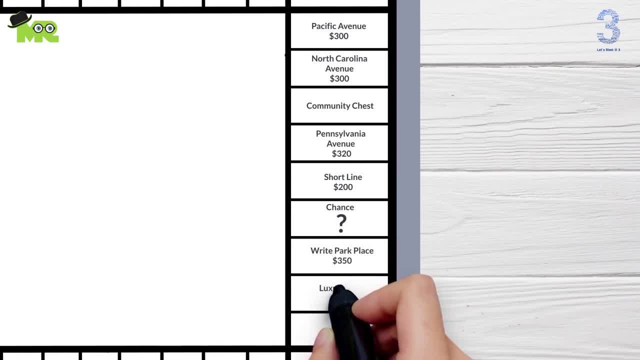 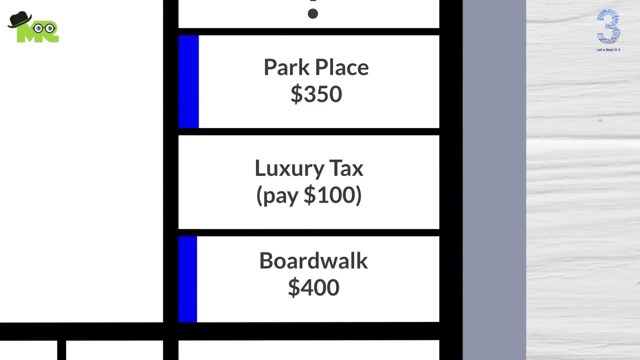 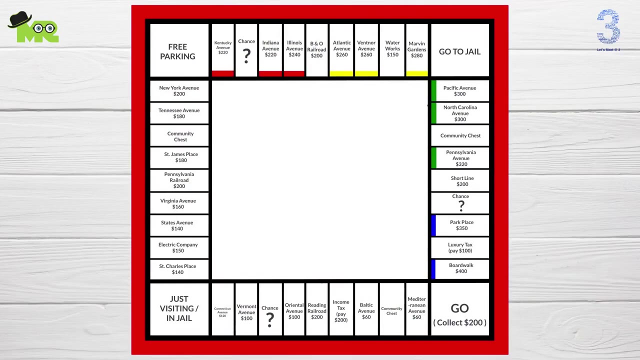 Park Place: $350, here And New York Avenue: $300, here North Carolina Avenue: $300, here And County knock, buy $1.. She Zarinp situations and go: green here, Blue, here Yellow, here Red, here Orange, here Purple, here Brown here. 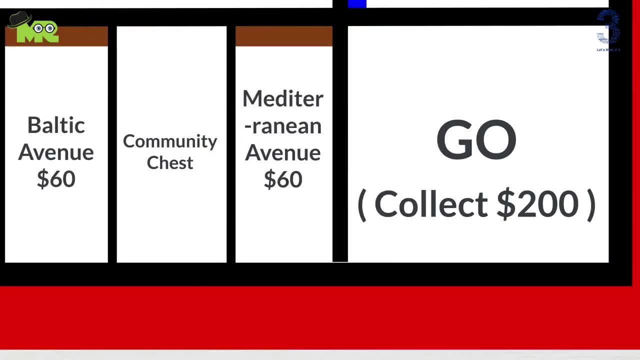 You can see it now. Know where Is that number Looks good. we may just do it here. That's impressive Pump. Hello, that's perfect. I need to get to do A very good ass blue here. Which one would you like to do?